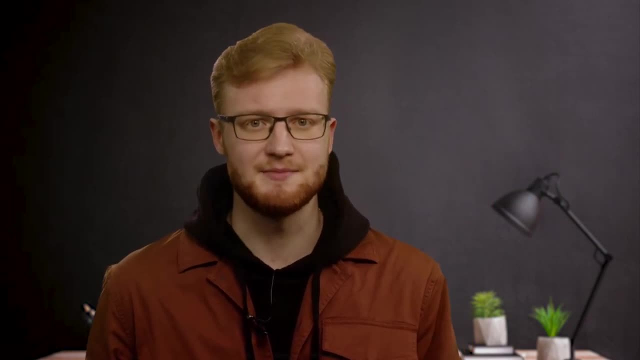 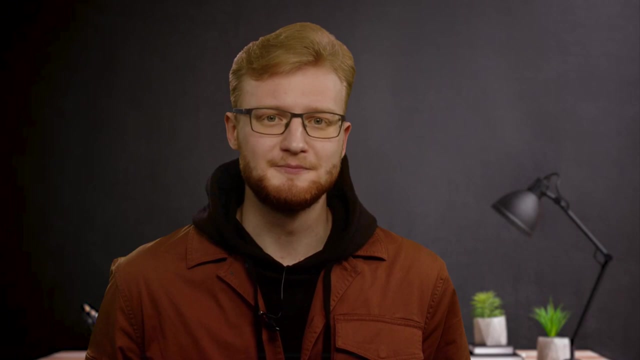 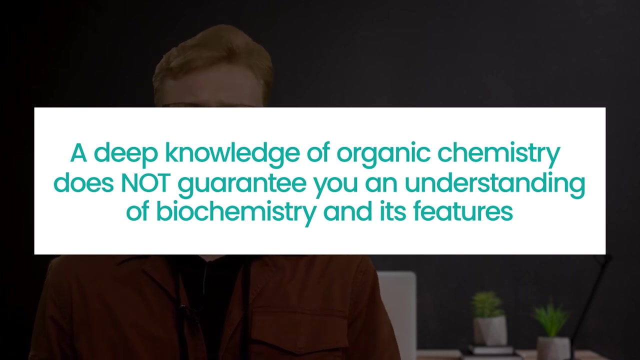 subjects, which remains with you until the very end of your studies. The more important question is – what is the practical demand of it? In this video, we are going to answer all these questions for you. And the main surprise from the very scratch – a deep knowledge of organic chemistry does not guarantee your understanding of biochemistry. 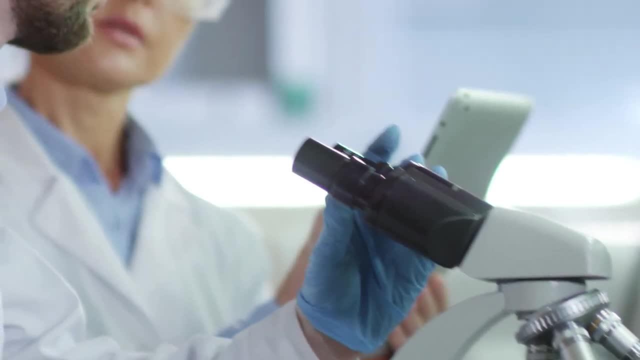 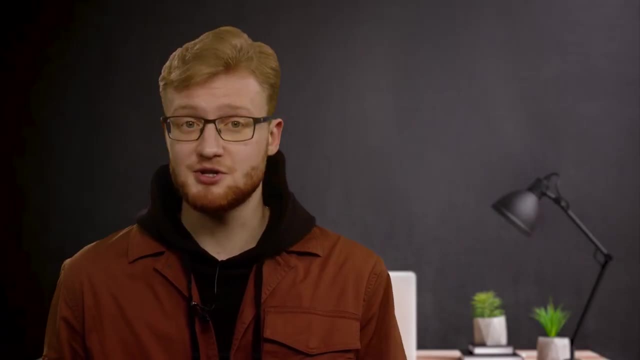 and its features. And here is why – over its more than 100 year of history- biochemistry has managed to become a completely independent study. It would be even wrong to perceive it as a branch of chemistry. It has its subject of research, its methodology, it generally 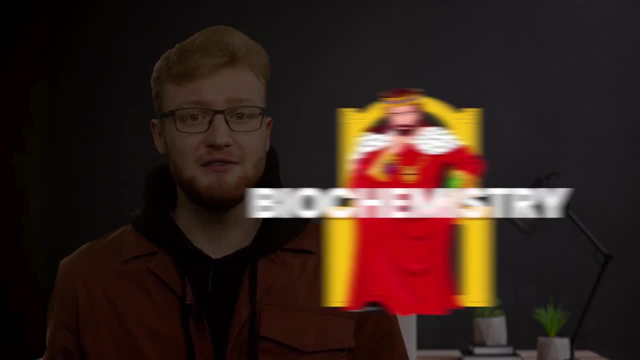 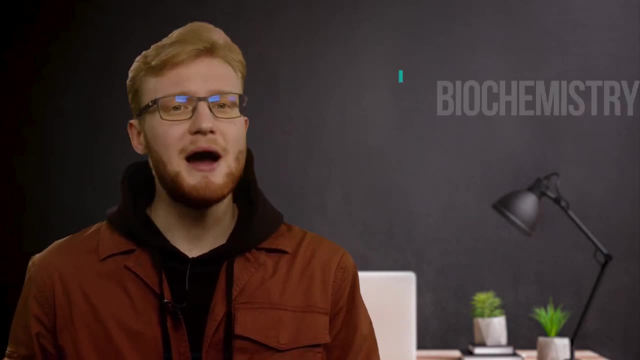 has everything of its own. You might ask – why is it so special and even diverged into a subject of its own? It's actually not diverged at all, but here you need to understand the main point – biochemistry is not the same as chemistry, Even the bachelor's degree. 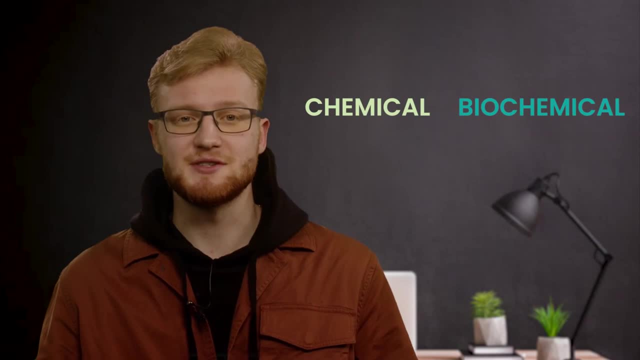 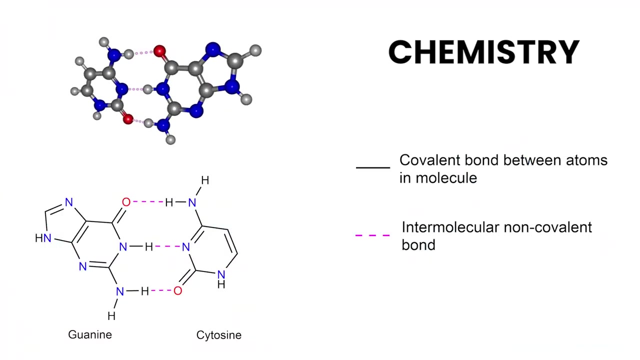 is often divided into chemical and biochemical sections because they are not just different, but different fields of studies. They are fundamentally different ways of thinking. Classical organic chemistry is more about how strong the covalent bonds are between the atoms in molecules, And the main thing you will have to face in biochemistry are: 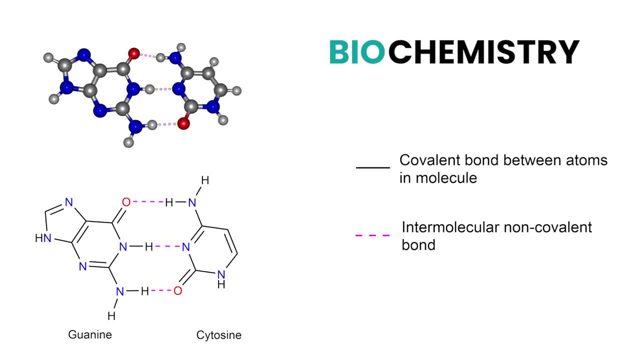 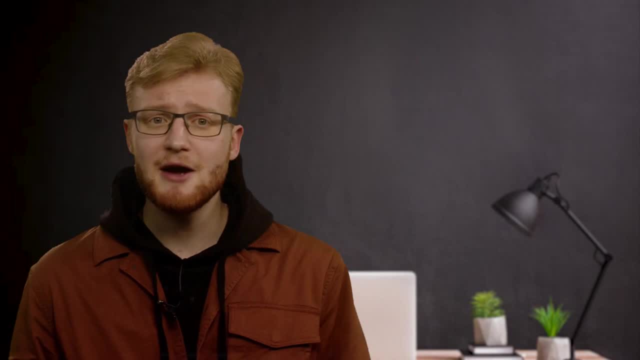 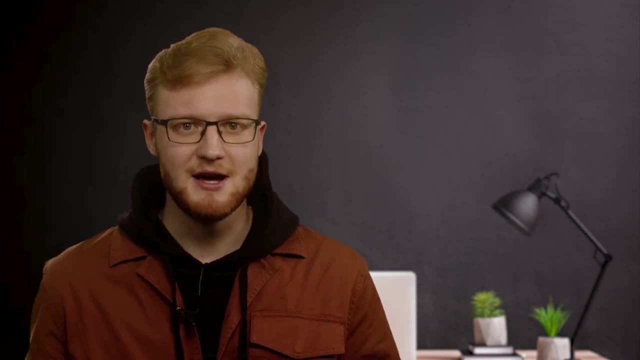 non-covalent intermolecular interactions between the macromolecules. And here is where the fun begins – this all happens inside living organisms. As a result, biochemistry not only becomes a subject of its own, it also consists of content from disciplines, For instance organics. you can't get away from it. cell biology, biophysics. 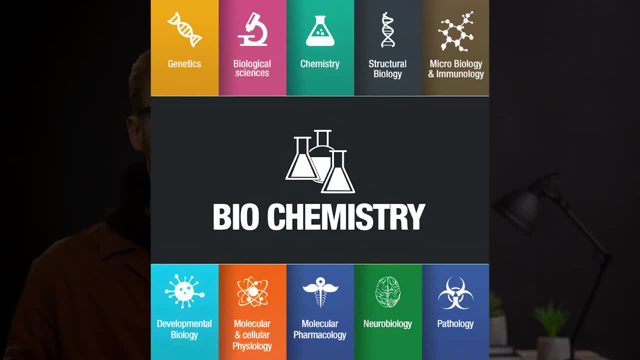 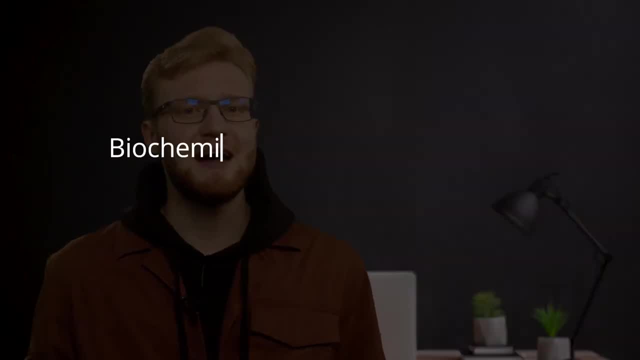 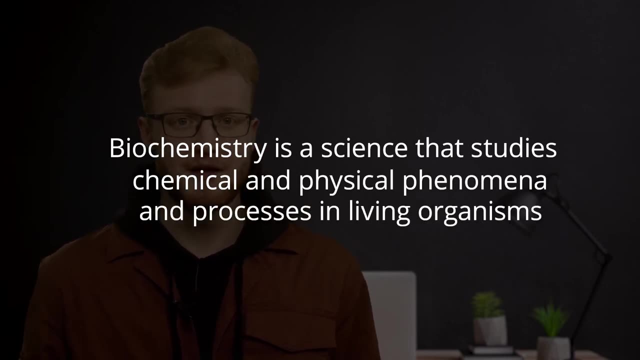 supramolecular chemistry. Biochemistry also has its own experimental methodology. So what is biochemistry? without going deeply into details, Biochemistry is a science that studies chemical and physical phenomena and processes in living organisms. This is very generally speaking. However, if biochemistry is such a specific subject, why do we chemists? 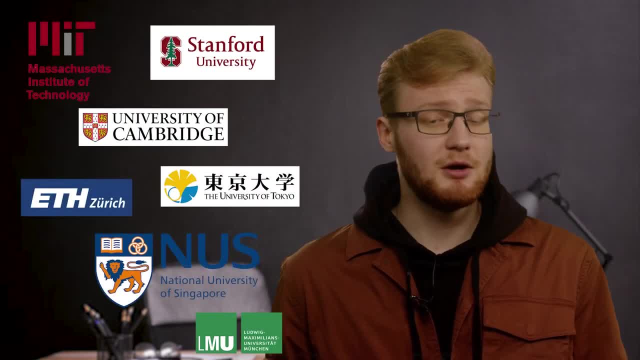 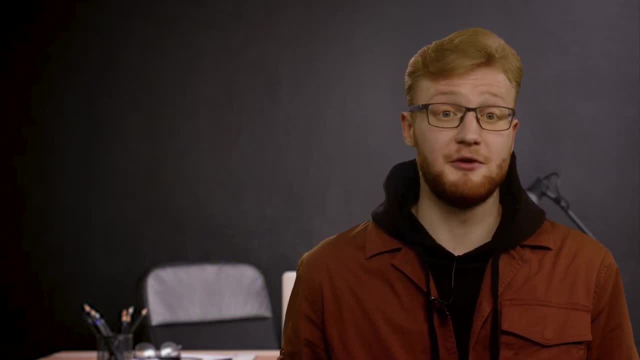 need it at all. The thing is, the world's top universities have long come to the conclusion that all chemists, without an exemption, do need biochemistry. Of course, this has to do with the further application of this knowledge, And we can say with complete confidence – if your job. 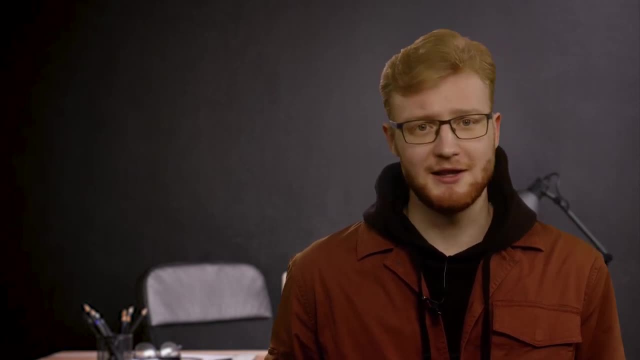 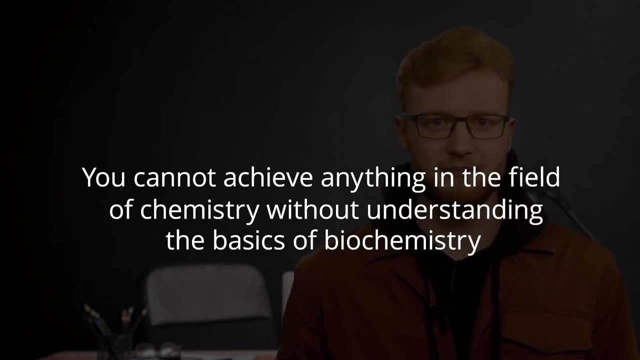 has anything to do with chemistry. biochemistry will not leave you alone. You cannot achieve anything in the field of chemistry without understanding the basics of biochemistry. When I finished my fourth semester of bachelor's studies in Munich, I had an internship in the University of Bavaria, where I studied biochemistry. I had an internship in the 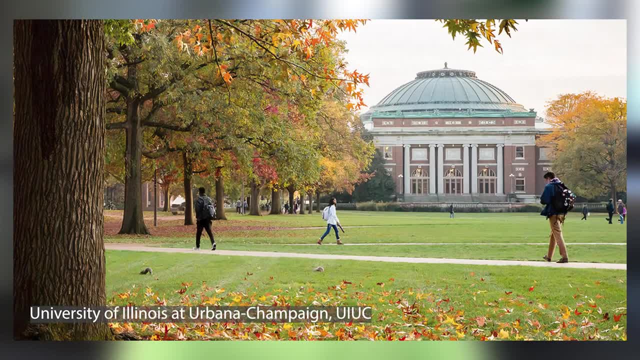 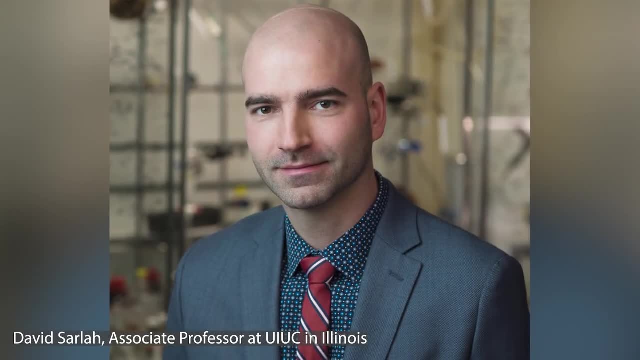 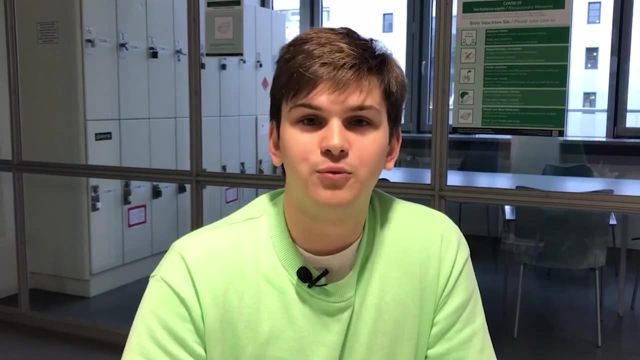 US in the UIUC University in the group of Professor Dr Sarlach, And this group is dealing with total synthesis of huge organic molecules. But I was personally involved in the project in this group that was dedicated to the high-throughput synthesis of small 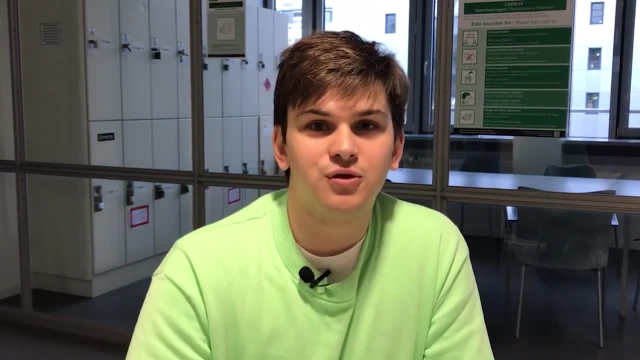 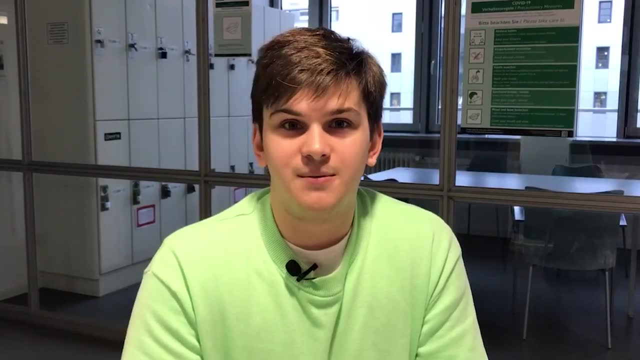 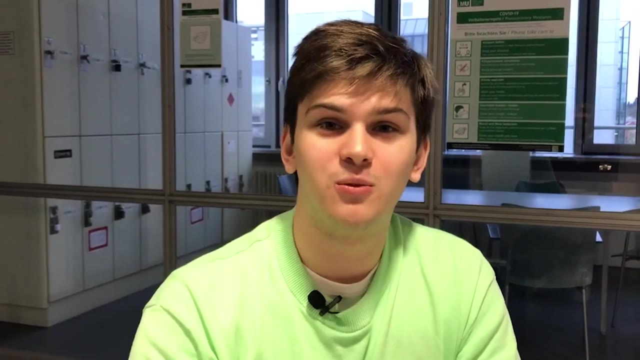 organic molecules that are the possible targets for the future drug design. And this is a perfect example of how the organic chemistry research, the fundamental organic chemistry research, is valuable for the biochemistry. Actually, there are many examples how biochemistry can benefit from the fundamental research in pure chemistry fields. For instance, I 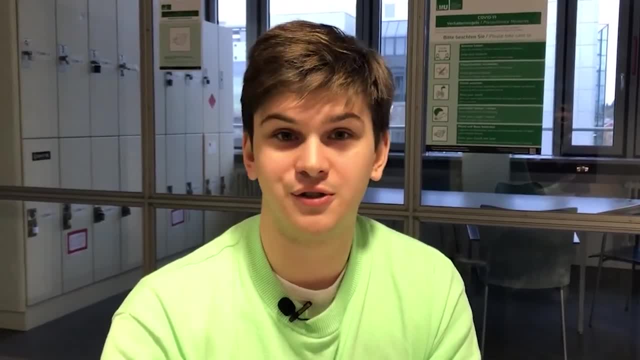 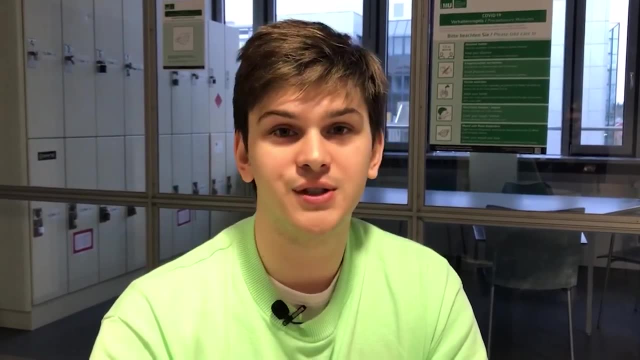 had finished my research internship in the group of Professor Nyssen, who is famous for his theoretical chemistry investigations. But my subgroup has dealt with Photosystem 2, which is the main component of chlorophyll, which is responsible for oxygen production in the world. 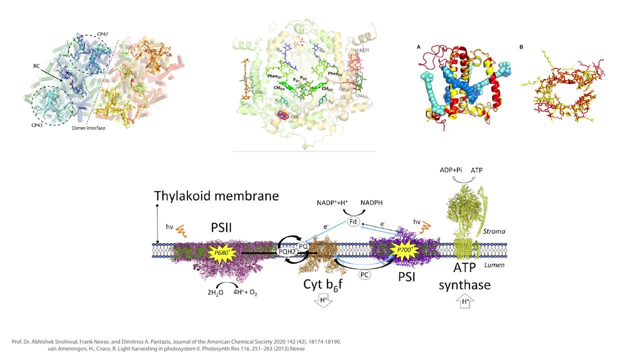 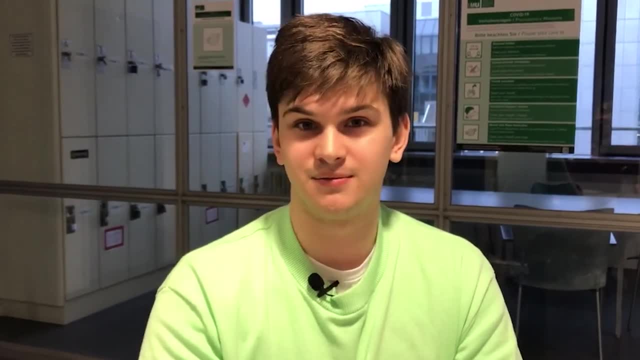 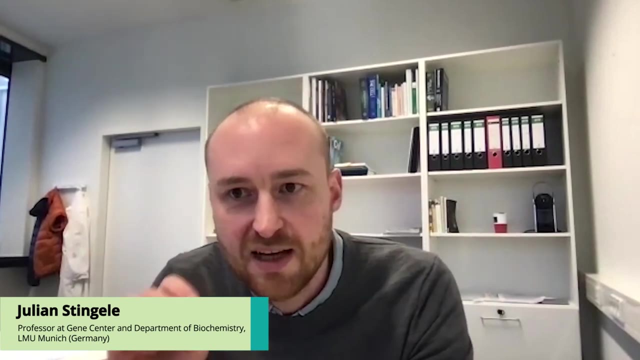 We have studied the structure and the mechanisms of how Photosystem II works, and this knowledge is vital when we are speaking about the synthesis of artificial photosynthetic systems. So we're not developing, let's say, universal laws, like a physicist might try, but the idea. 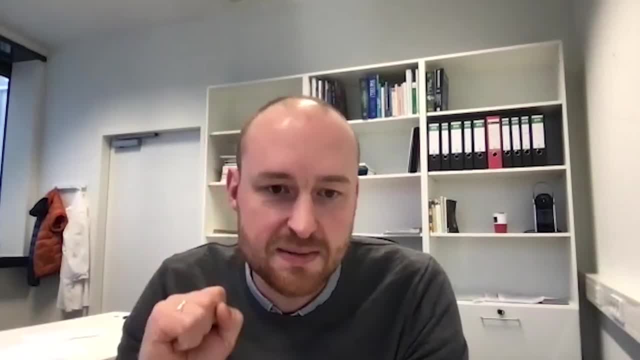 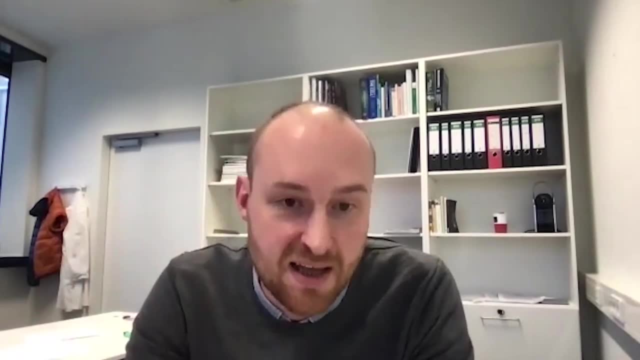 is to figure out regular principles and mechanisms which are true beyond that individual context in which you are studying it. And, of course, this has implications to various aspects of biotechnology, disease, biomedical research, And I think in this context, it's probably also worth mentioning that biochemistry is. 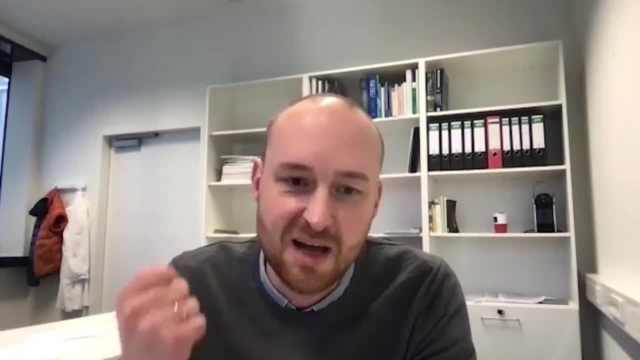 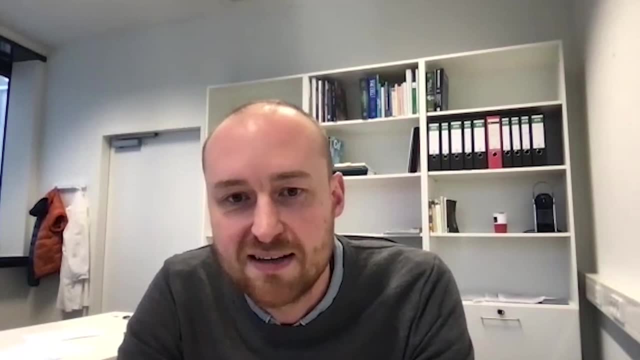 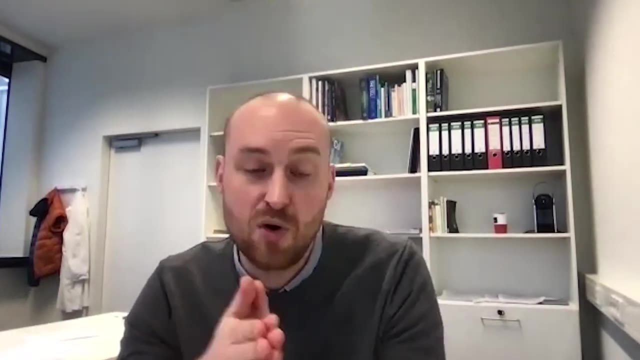 not an isolated discipline right where people train to become a biochemist and then you are a biochemist for your entire life. Maybe that was true 40,, 50 years ago, but every biochemist uses molecular biology techniques. Some of biochemists are maybe more at the intersection with chemists. 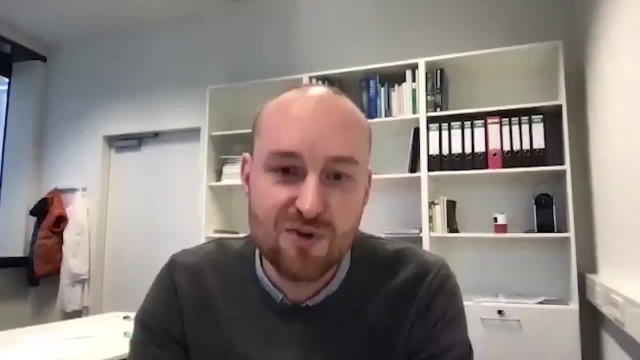 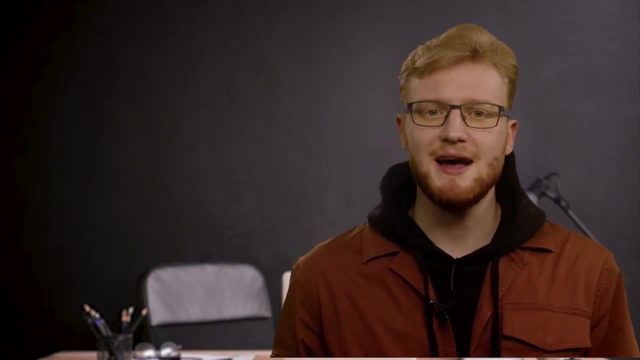 But a lot of work at the intersection with biology, neurobiology, genetics, immunology. There is a logical explanation for the popularity that biochemistry has, and it's not only related to the development of this field itself, but also because of the people who are generally 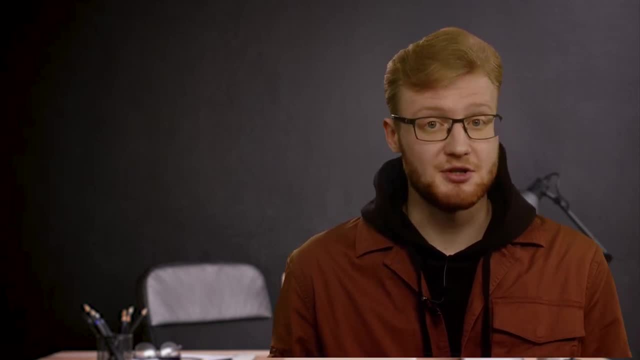 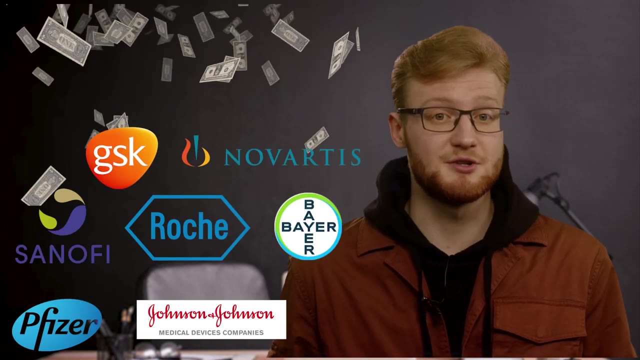 interested in not only their nature, but also in the preservation of their own health. That is why a lot of money and time is invested now in biochemistry and pharmaceuticals researches. Nowadays, Biochemists are a kind of hype And, yes, hype is also very welcomed in science. 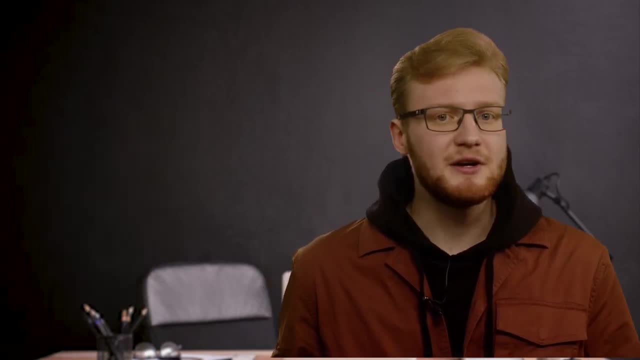 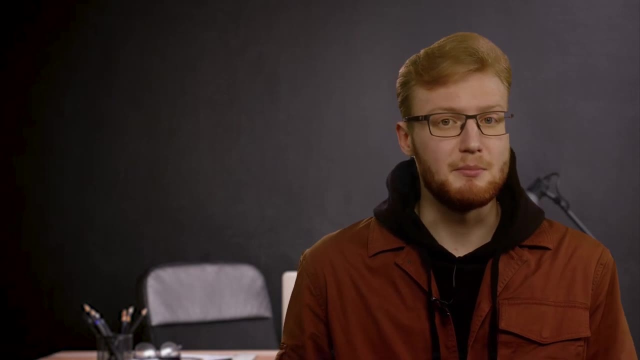 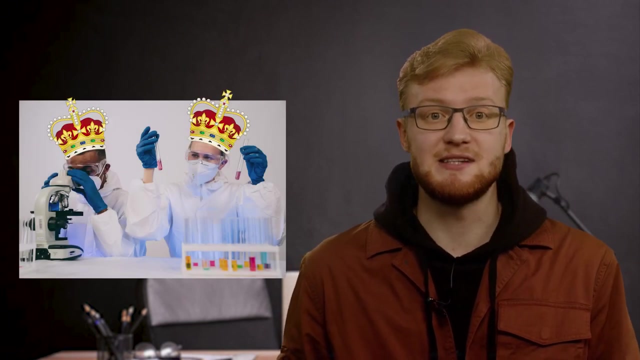 So this creates a whole trend in global research. Therefore, even in the other fields of studies that have a slight similarity with biochemistry, the researchers try to comply with it. meaning, at the stage of formulating research questions, topics and themes, researchers try to somehow select them so that they satisfy the needs. 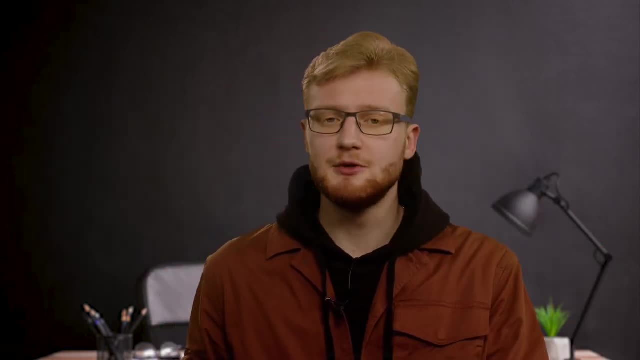 of biochemistry. Just to give you some good examples, here are the Nobel laureates of recent years. A number of them received their awards for their work in biochemistry. The Nobel laureates received their awards for their work in biochemistry. The Nobel laureates received their awards for their work in biochemistry. 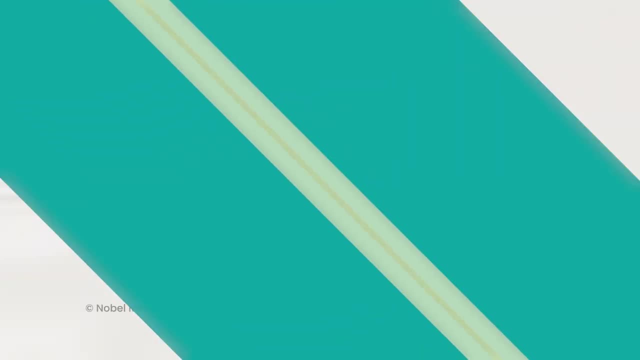 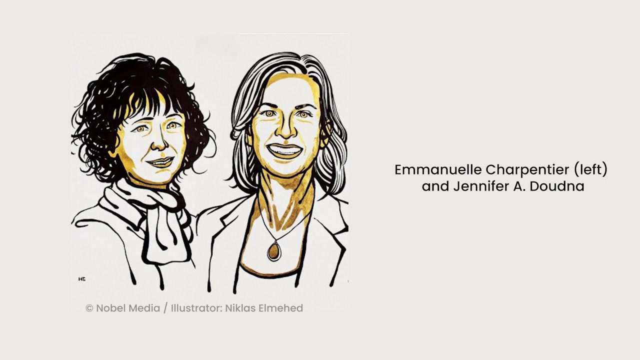 They won the Nobel Prize for the application of the results in the field of biochemistry. Like Emmanuelle Charpentier and Jennifer Doudna, both received a Nobel prize in 2020 for their contribution to their own invention made in 2012.. 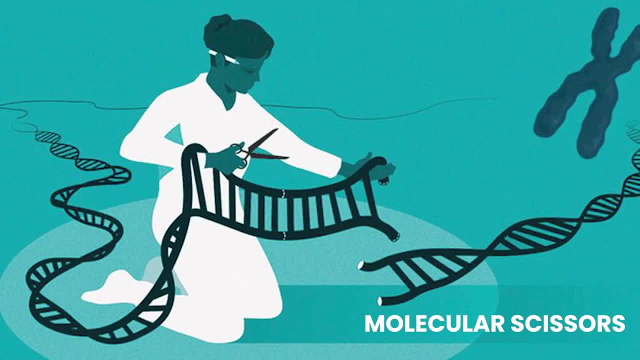 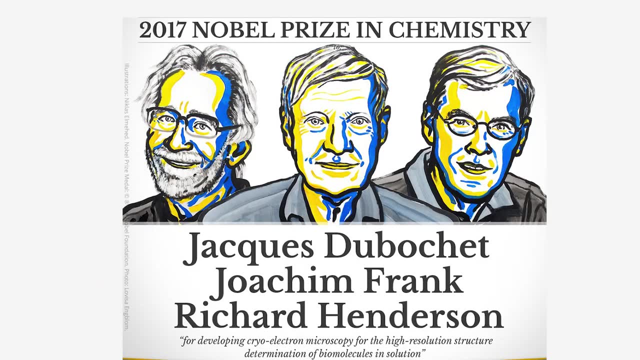 I'm talking about molecular scissors which will help create new treatments for cancer as well as hereditary diseases. And here's another example: Jacques Duboisier, Richard Henderson and Joachim Frank received their award for the development of high-resolution cryo-electron microscopy. 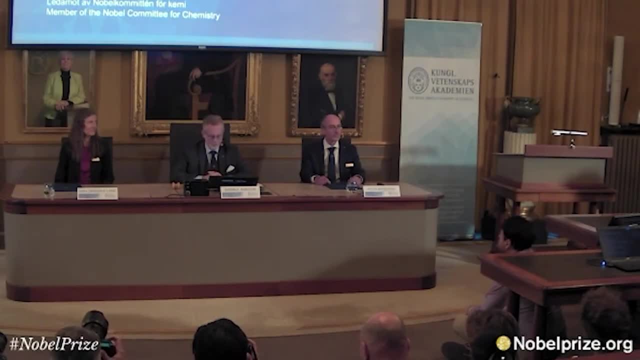 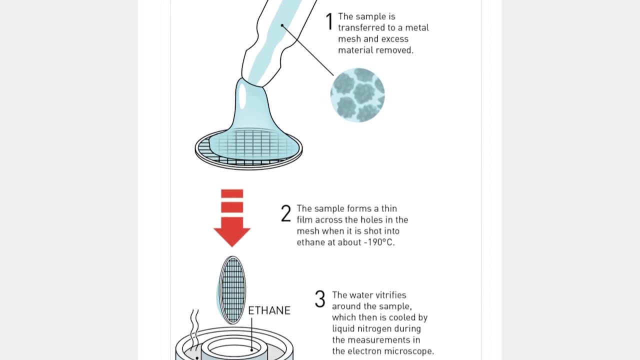 received about 1 million euros from the Nobel Committee for this. In simple words, these people have invented technology that has brought us closer to understanding the very essence of biological processes. Long story short. thanks to it, researchers are able to freeze biomolecules. 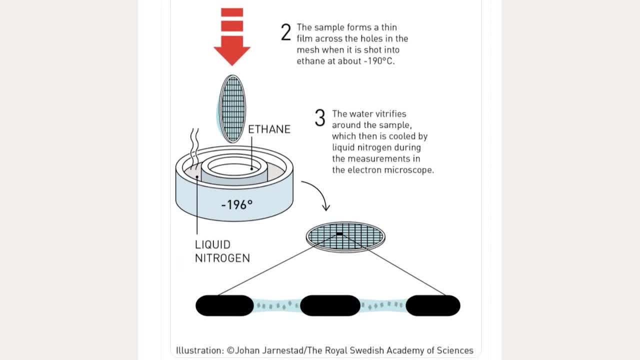 mid-movement and visualize processes they have never previously seen. So it enhances our understanding of how this or that pill works and whether it's possible to invent something better. And perhaps an example that many are hearing now: the Nobel Prize for Asymmetric Catalysis. 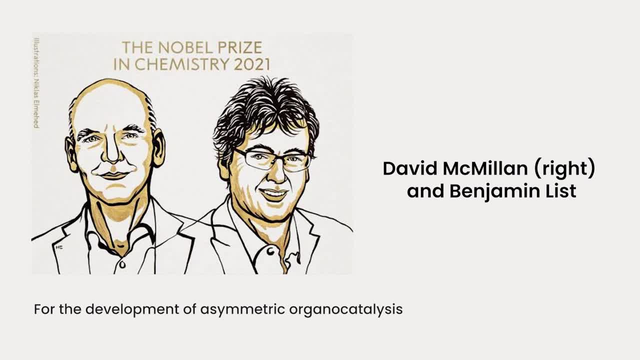 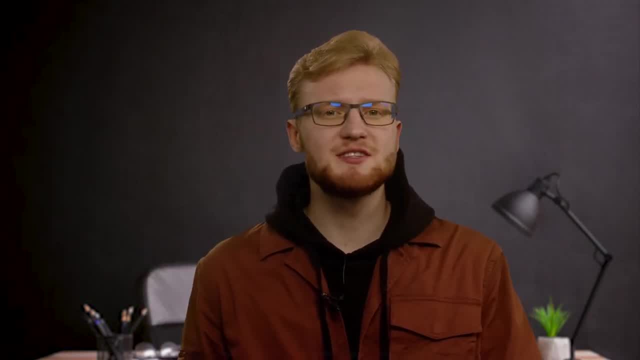 David Macmillan and Benjamin List were honored for inventing a catalyst that makes medicines without side effects and without polluting the environment. So, as you may see, biochemistry is really kind of booming branch. What is it studying which is so important that humanity desperately? 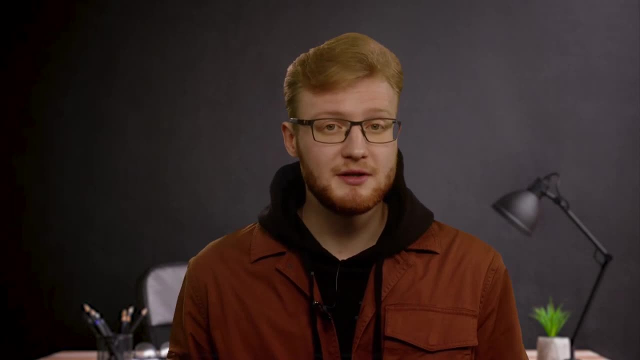 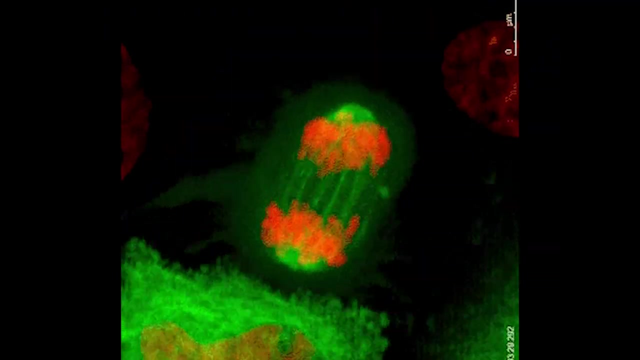 needs it. Biochemistry tries to answer the most important questions about how the living organisms function. Where did life come from? How did it come to be, How did it come to be, How did it come to be, How does it reproduce itself, And what is death? The last one is actually a much more tricky. 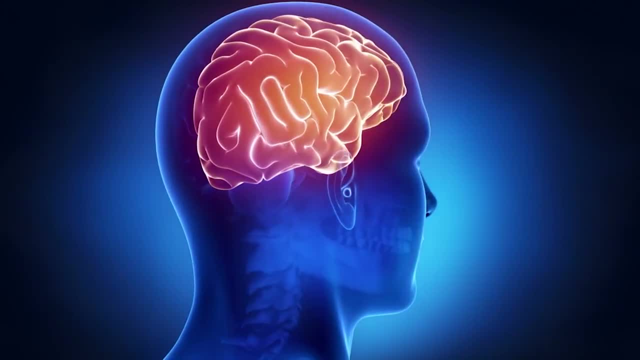 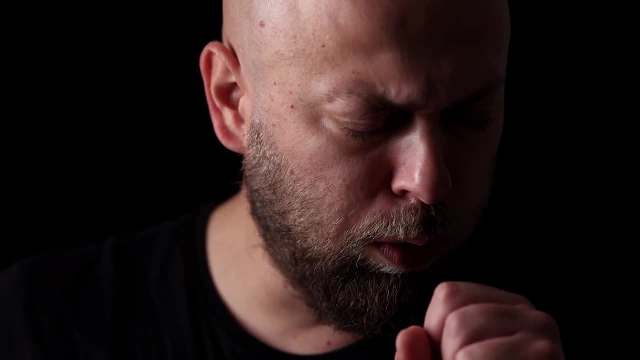 question, as you may think: How does the human brain work and why do we experience different emotions? Why are we getting older Or, for example, getting sick with something, be it cancer or coronavirus, And, most importantly, can we people influence any of that? We asked a biochemistry. 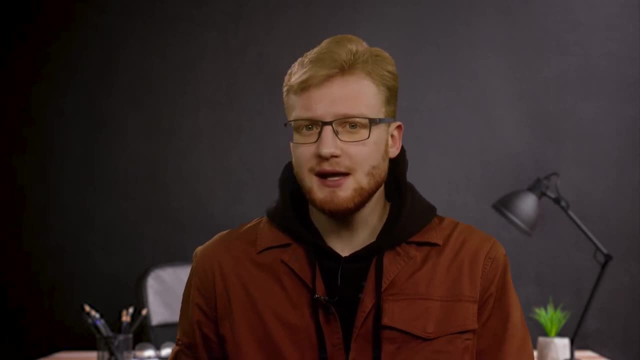 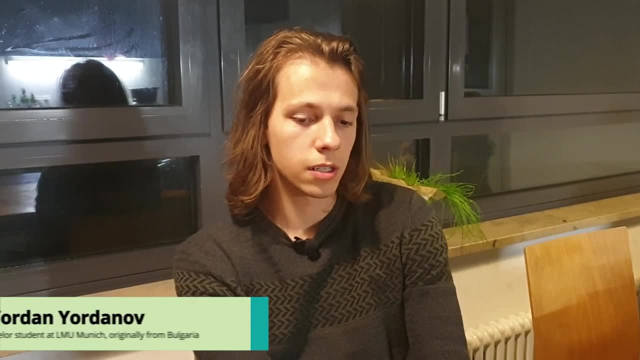 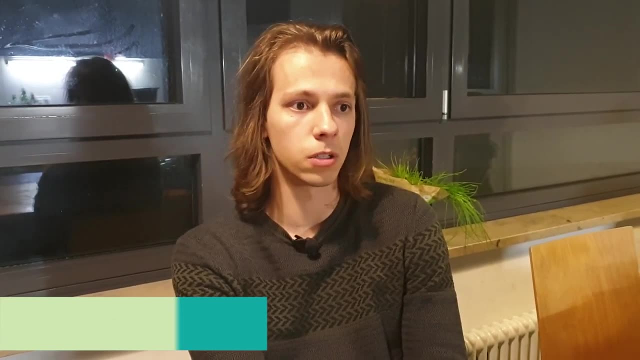 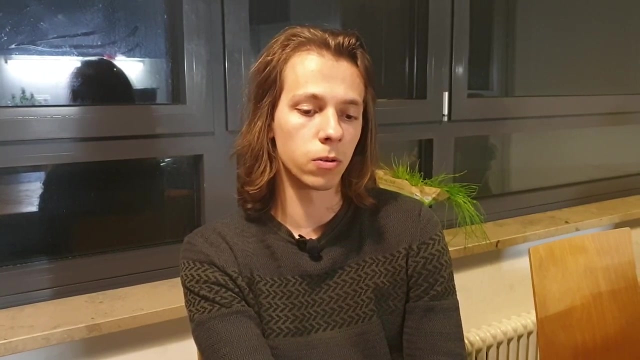 And that's what he told us. At the moment, chemical research is really very much oriented towards biochemistry. You can do things like bioorganic or bioinorganic chemistry and vice versa. With theoretical chemistry. you can also calculate structures like biomolecules and so on. As part of the bachelor's degree at our university, there are 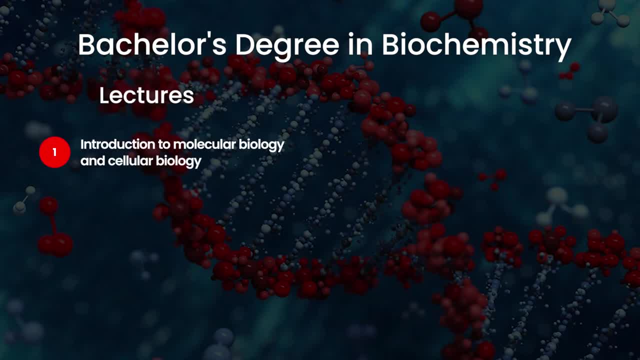 three lectures on biochemistry. Name: Introduction to Molecular Biology and Cellular Biology: Foundations of Metabolism, Enzymology and Drug Development. Advanced theoretical aspects of protein biochemistry. Practical lab course for biochemists where typical basic experiments are carried out, such as how to do a PCR test, how to clone cells. 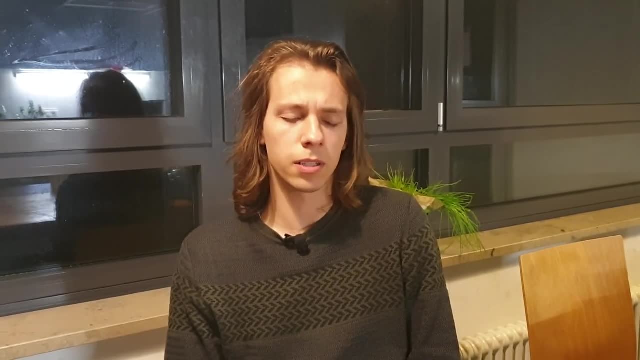 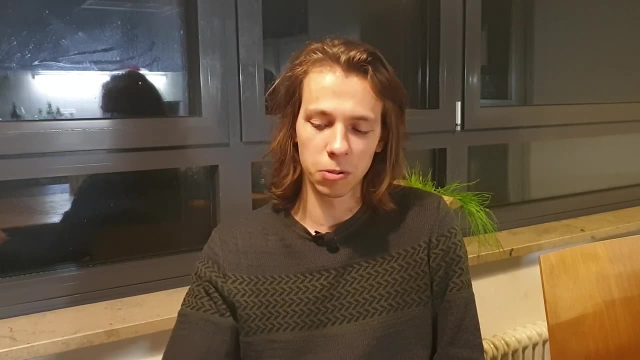 Of course, something exploded during our internship. It always happens in every internship that someone breaks something. We are students And, above all, we are people. We are not flawless. I would say you don't need that much previous knowledge, But the more previous knowledge you bring, the better. 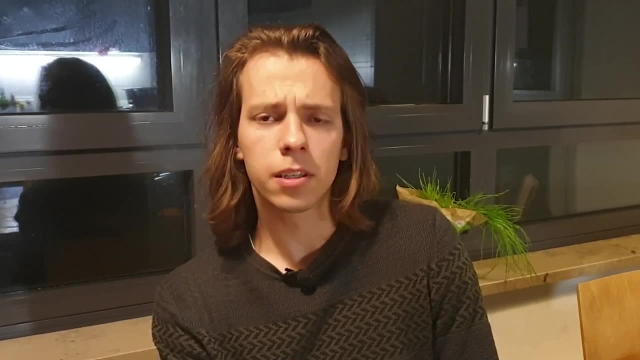 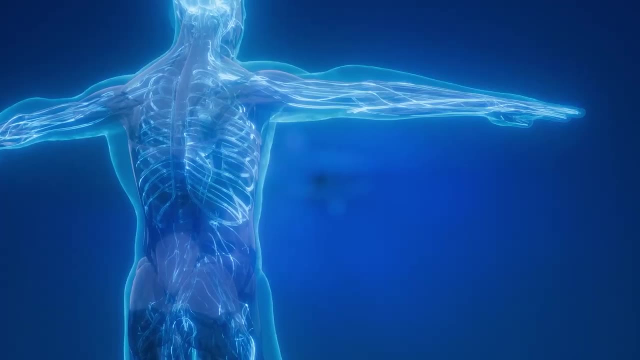 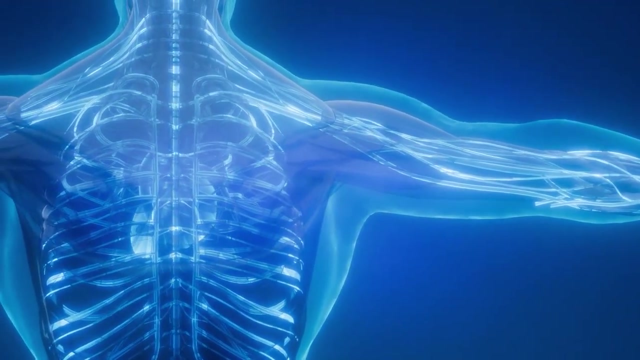 That was mainly previous maths knowledge, But also various things in chemistry. The people who are interested in biochemistry are usually more interested in metabolism and everything related to the human body and human cells. But it's not just about metabolism, although metabolism and physiology are of course, also very interesting. 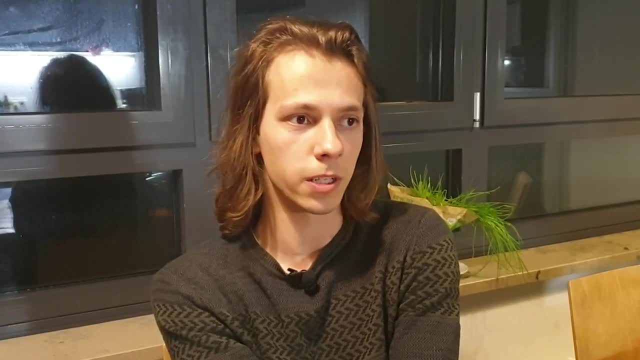 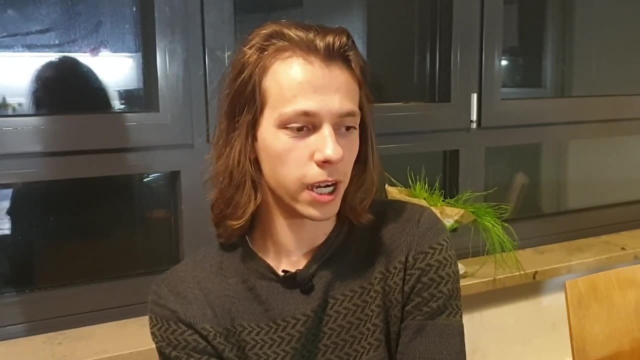 But it includes more things: Genetics, cancer development and generally studying different diseases. So you shouldn't think that it's just about diets, metabolism and so on. So for people who are up for medical things but still don't want to study medicine as a medical thing, then you can be interested in biochemistry. 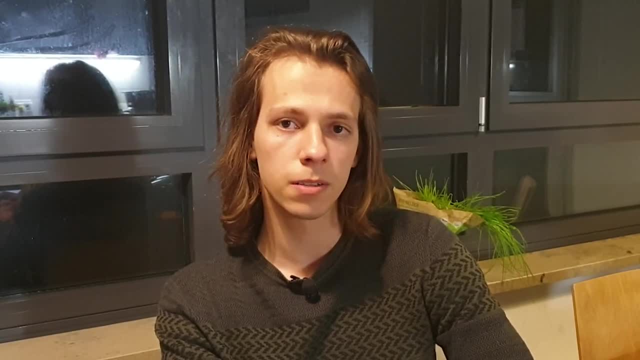 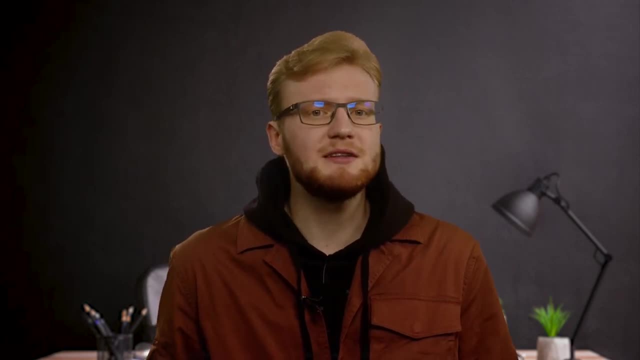 a subject I would highly recommend: biochemistry. Okay, let's say you became graduated biochemist. What can you do with that? What are your prospects? What can you do later if you are well versed in such a tricky field as biochemistry- And here you have a great deal of 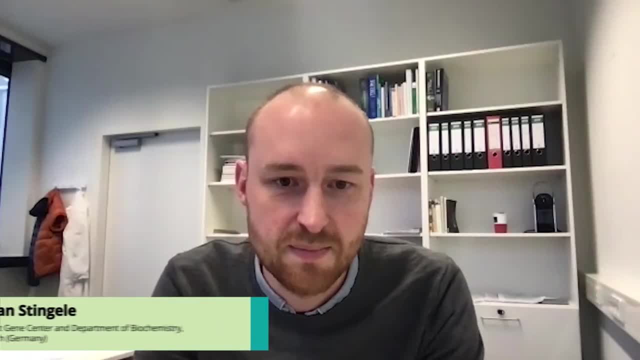 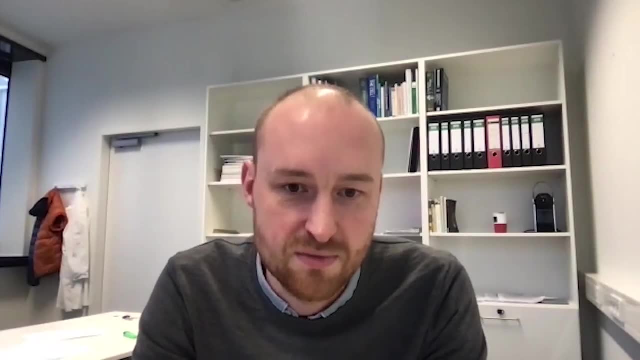 different fields and professions to choose from. I'm a biologist by training and then I did my PhD at the Max Planck Institute for biochemistry and I then moved to the UK for postdoctoral research. I returned to Munich then as a tenure-track professor. 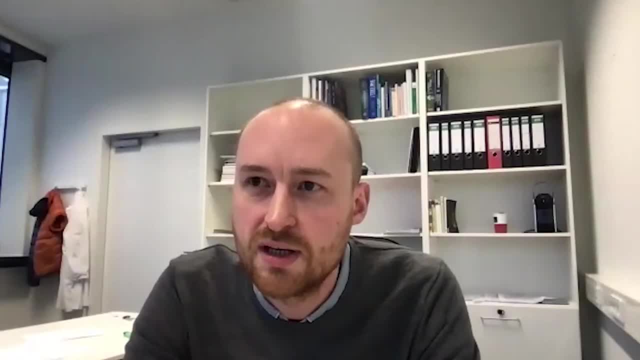 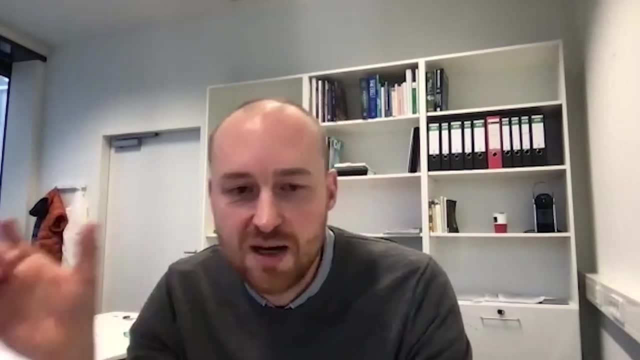 here at the Gene Center for cellular biochemistry. What I really enjoyed in high school in the final years was learning about molecular biology, about you know how a gene is transcribed into mRNA, how that is then translated into the protein. I've been 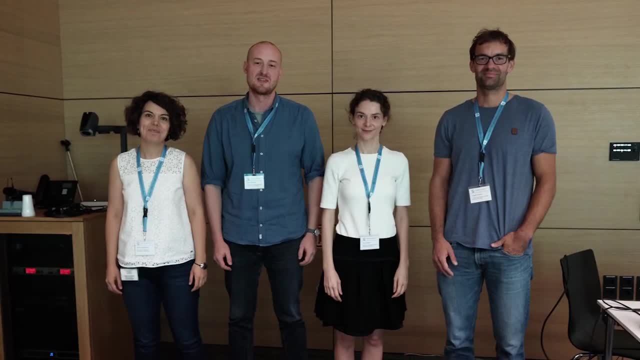 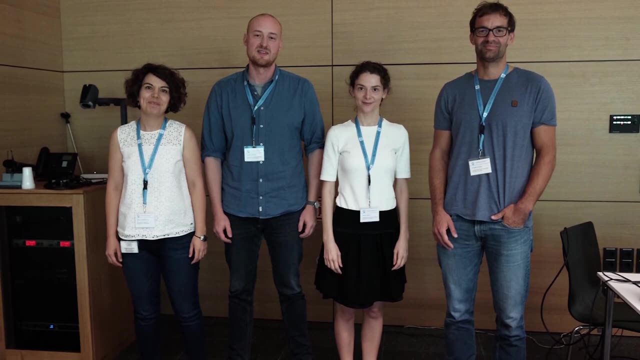 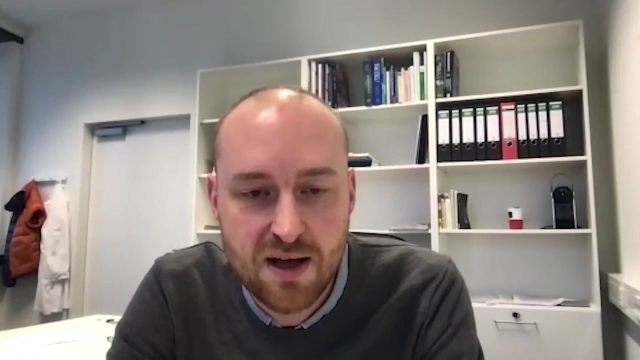 running my lab here now since roughly four years and I teach courses in the Bachelor of Chemistry and Biochemistry and also in the Master of Biochemistry um program. We are interested in DNA repair, So the DNA in all of our cells encodes the genetic information. 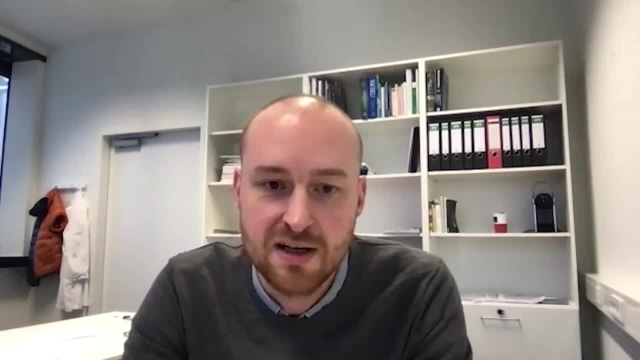 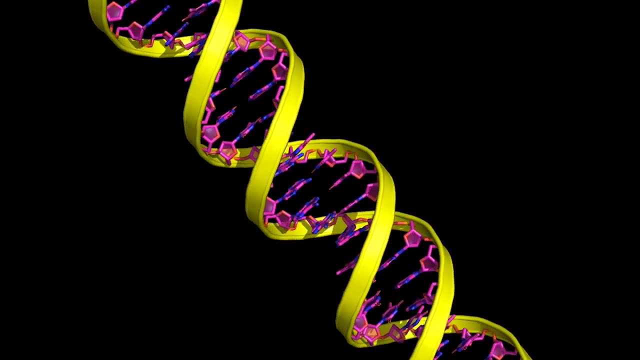 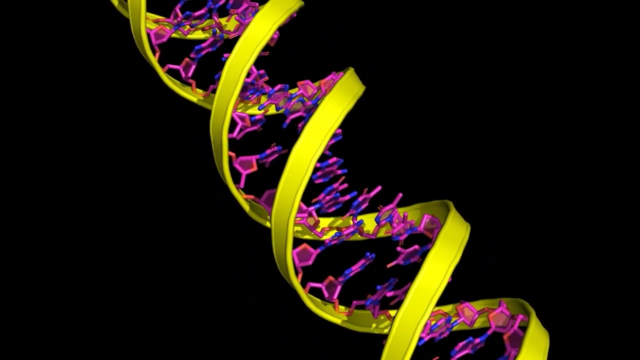 and this information is permanently threatened by damage, For example, by UV light, but also by reactive metabolites- reactive agents produced by our own metabolism, which change sequence and structure of the DNA molecule, And it's very important for cells to detect these damages and repair them. 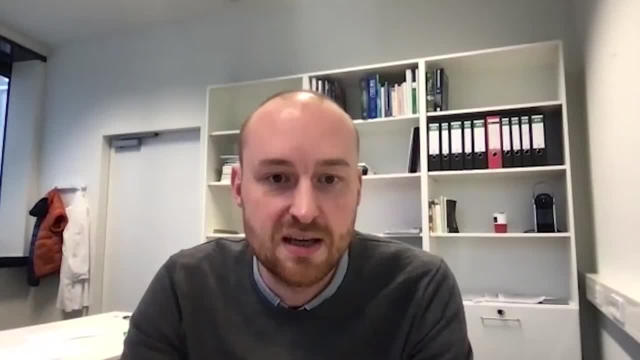 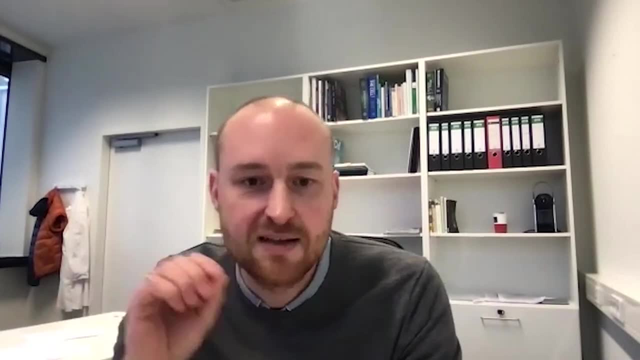 because if it fails, this, you know, can cause aging, It can cause the formation of tumors, the formation of cancer. So we're trying to identify all the factors, the proteins in our cells which are involved in this process. So enjoyed a lot because 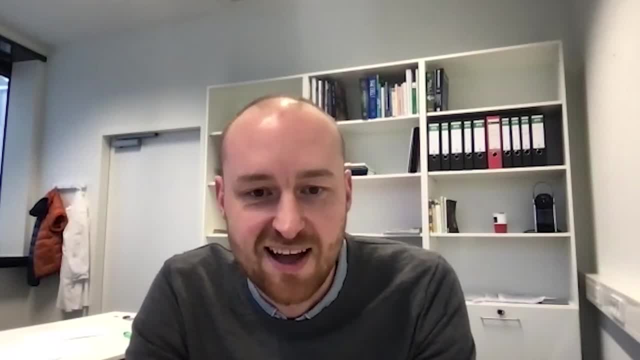 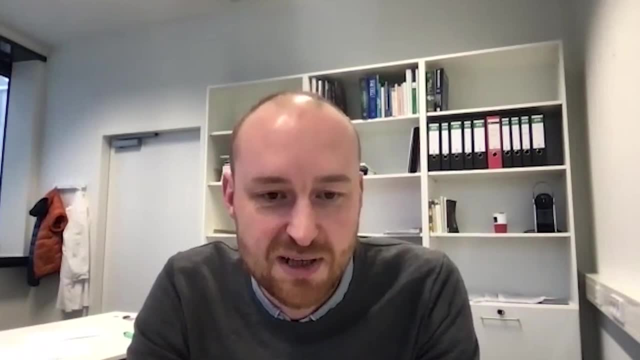 you know you can work with motivated young people and you know it's quite a thrill if they experience for the first time to figure something out on their own. And of course, it allows also me to follow much more interest. right, We can run ten projects in parallel and there is always you. 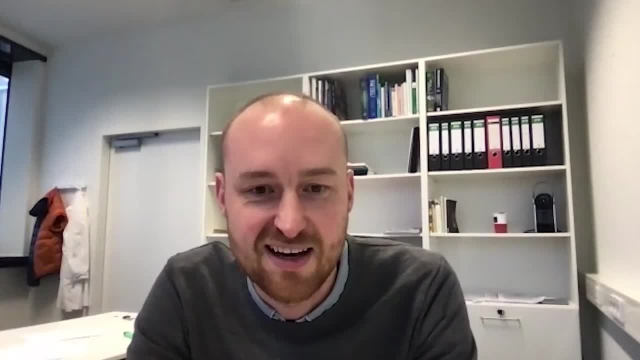 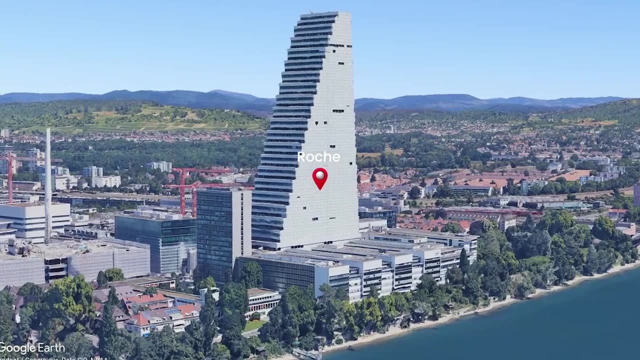 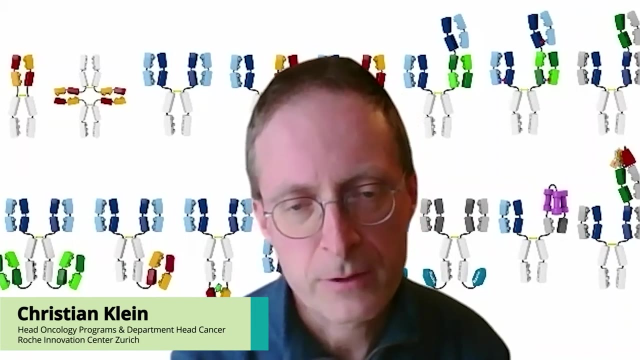 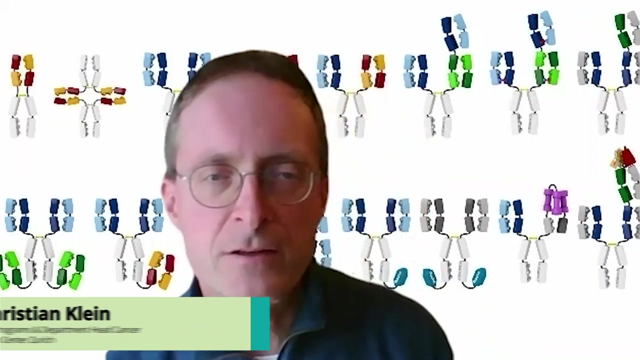 one which you know where is exciting stuff going on, and so i enjoy it a lot. i have studied biochemistry in tübingen and then for my doctoral thesis, i went to the max blank institute of biochemistry in munich, collaborated at the time already with rosh. in 2010, i joined the rosh. 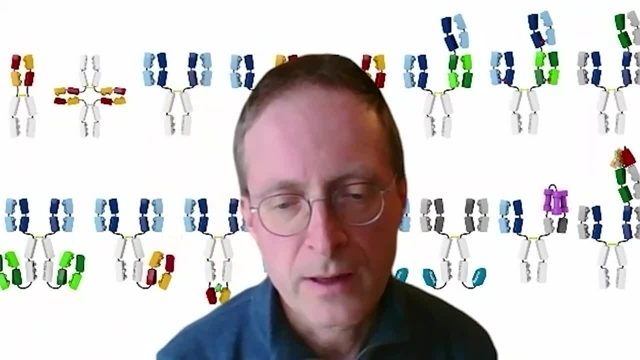 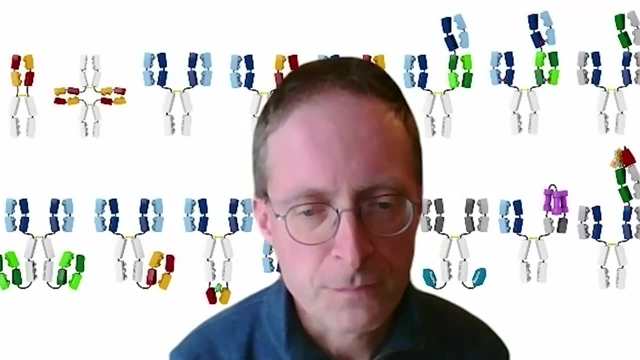 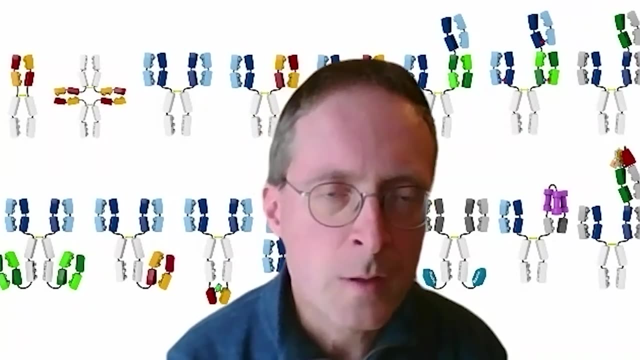 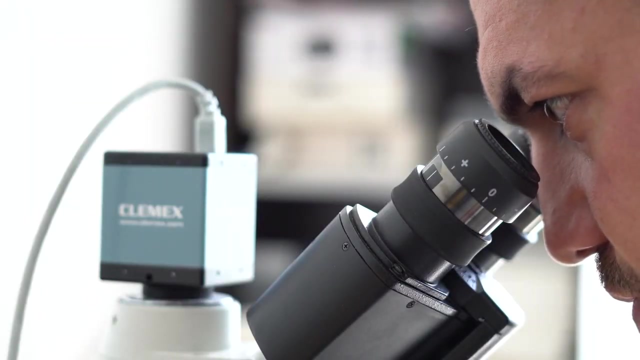 innovation center in zurich to work on cancer immunotherapy. so we are developing their bispecific antibodies for immunotherapy. we are doing this from the early stages- really the discovery- and to moving these molecules forward into into clinical development and i are confident that also some of those drug candidates hopefully in the future will be, will be. 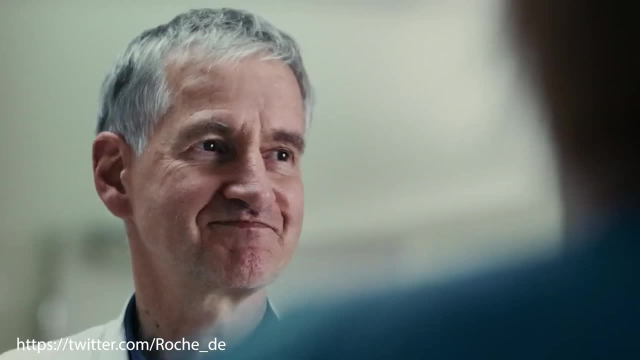 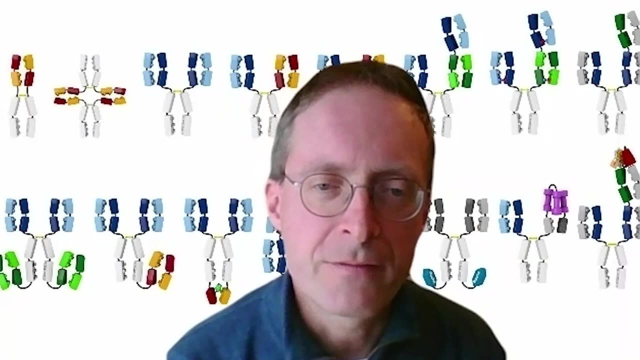 used in the future in the clinical setting. yeah, at rosh i think we do a lot of research. that that you maybe could also find in an academic environment, but of course the focus is a is a little bit different in the sense that, yeah, we really have the purpose of developing a drug candidate that can enter into 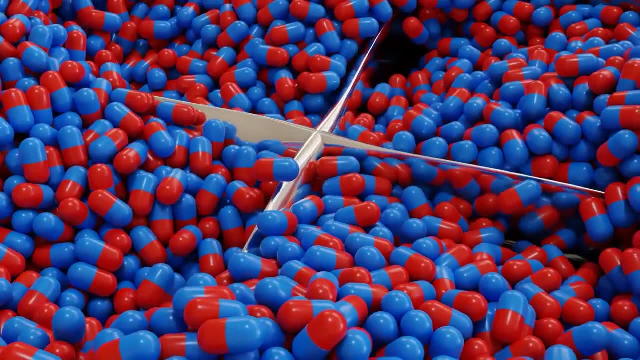 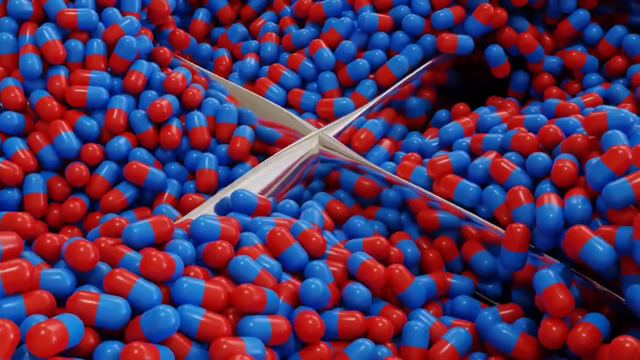 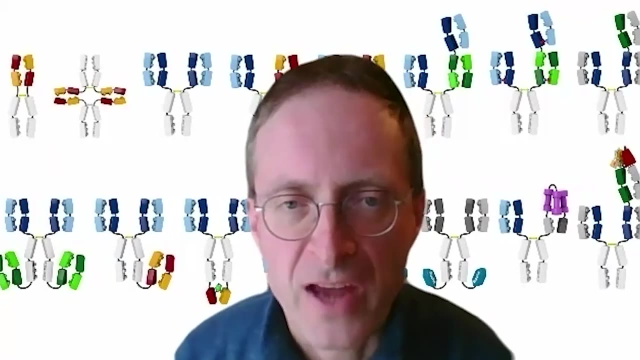 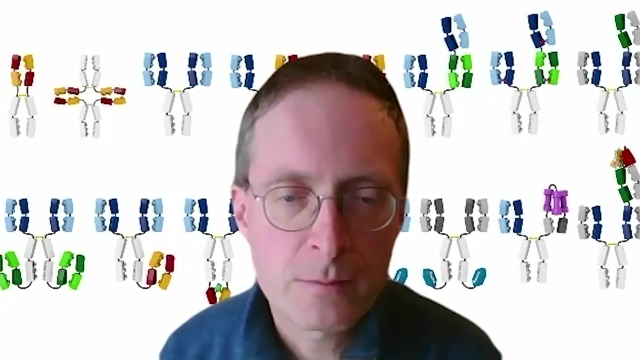 into clinical trials and hopefully come on the market. so we, we do applied research really with the, the, the the purpose of drug discovery, of course. now, all all our people, they, they have worked in in academia before and for our scientists, you know the majority of those- well, either has done a postdoc. 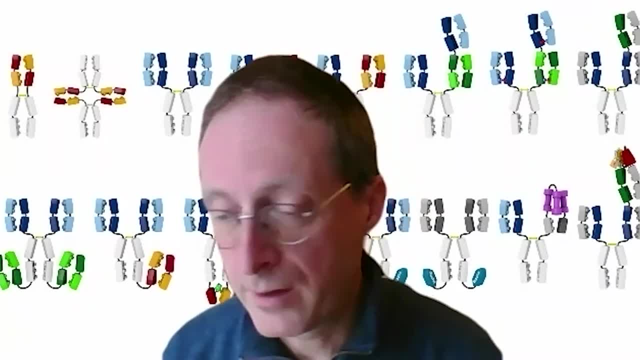 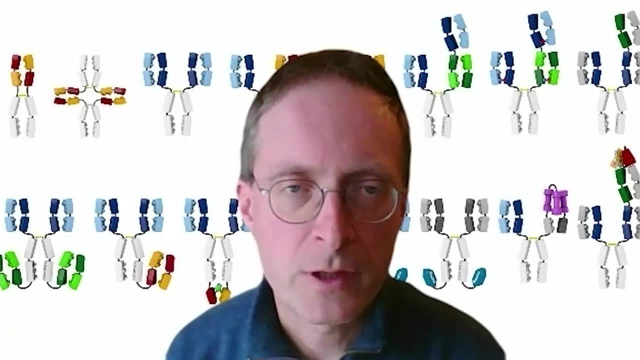 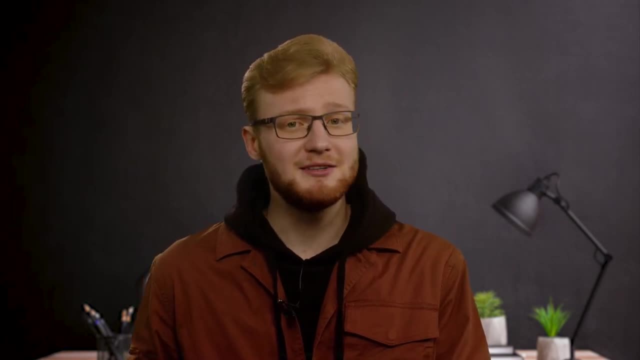 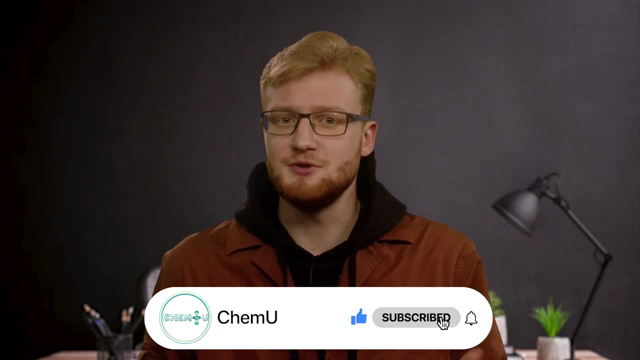 before there may also, or they even come also directly after their their phd, i think. i think typically we would rather hire somebody with a specific expertise we are looking for. well, i think typically we would rather hire somebody with a specific expertise we are looking for. well, i hope that we have given you guys a couple of insights and now you have a better understanding of what awaits you if you, after all, decide to study such a complex but necessary and even mysterious discipline as biochemistry. leave your ideas for the next videos in the comments. your likes are always most welcomed and you should definitely visit our chemical forum. you'll find there a lot of interesting things, more than you expect. see you soon. bye. you, you.